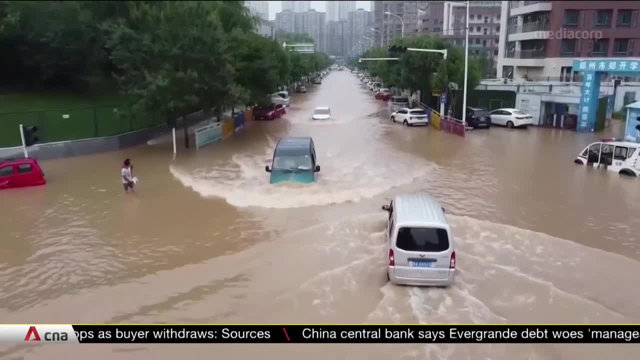 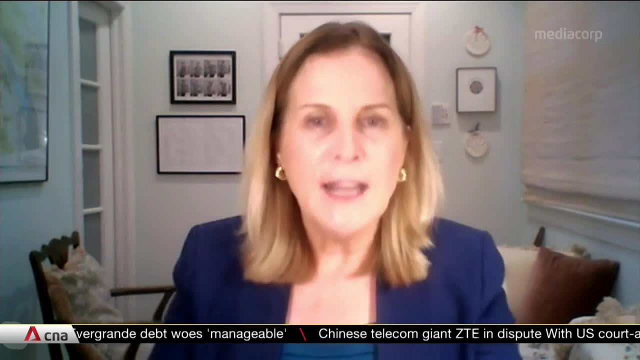 For climate adaptation, the role is to reduce the impacts and reduce the risks. For climate adaptation, the role is to reduce the impacts and reduce the risks, even if we succeed in our goals. it involves decisions across virtually every sector, every discipline. mitigation, on the other hand, has a very easy metric. 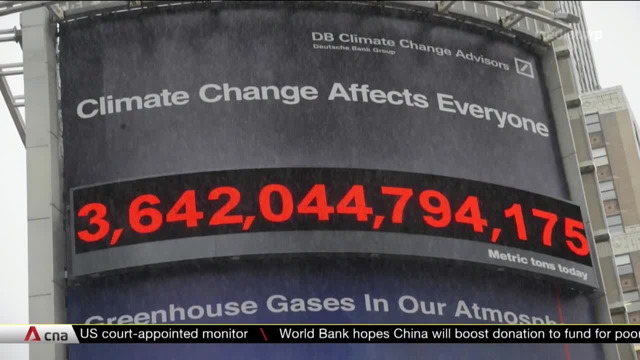 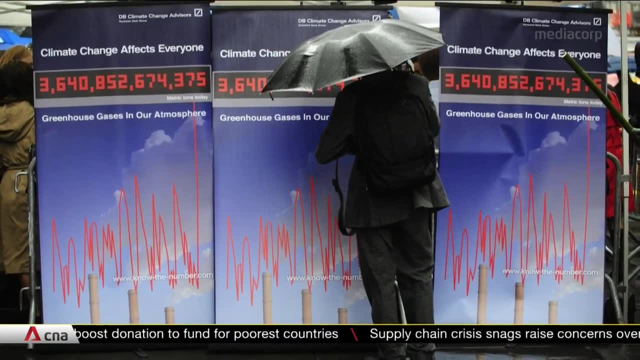 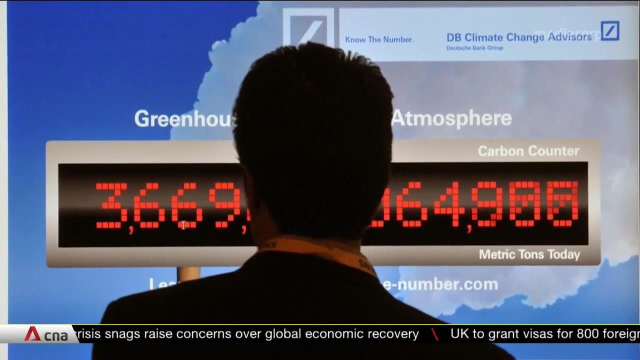 for measuring progress. how many gigatons have we kept out of the atmosphere of carbon? when you go back to adaptation, it is everything, and that makes it really hard to measure. but there is one measure that some might consider the most important: according to the UN's weather agency, the number of climate linked 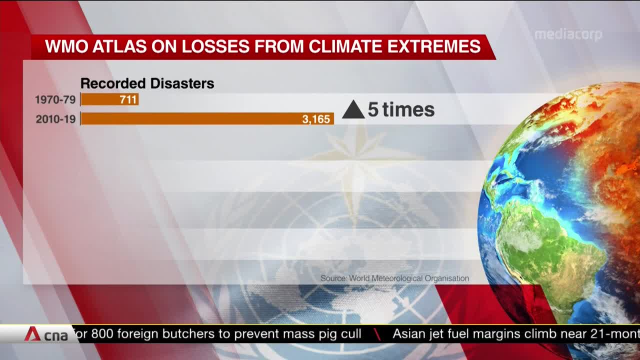 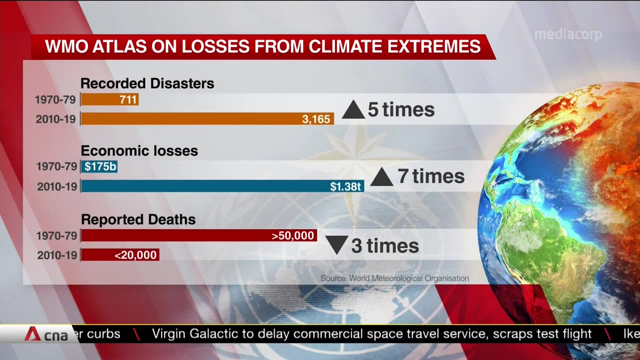 disasters has gone up five times in the last 50 years. the economic cost has also shot up a hefty sevenfold, but not so the cost in human lives. fatalities from extreme weather events have fallen almost threefold for the same period, as the head of the WMO puts it. 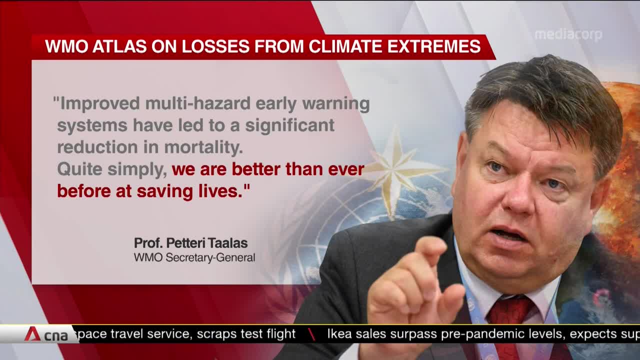 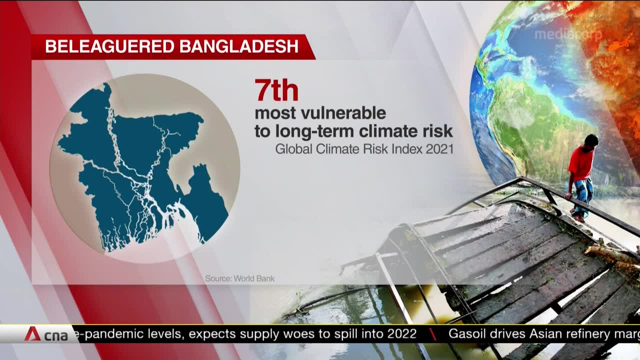 we have got better at adapting to save lives. that's something Bangladesh, ranked seventh in the world's most climate affected countries, has been forced, as a matter of survival, to learn. we are sitting on the Delta of two of the biggest rivers in the world, the Ganges and the Brahmaputra, which are regularly 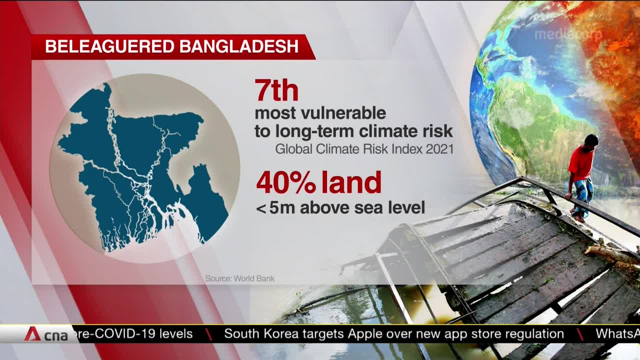 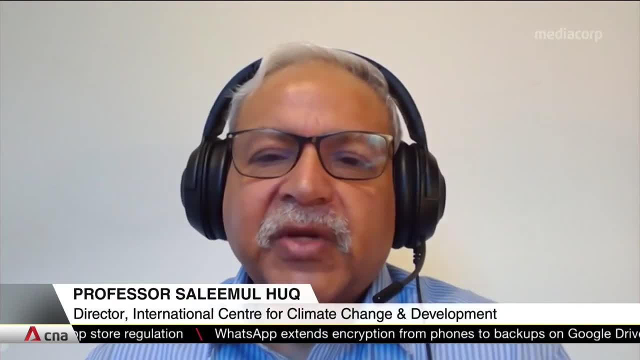 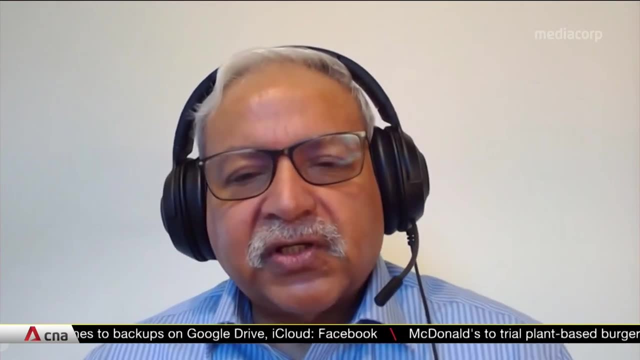 flooding. the other reason is that we have a very low-lying coastal zone which is susceptible to sea level rise and salinity increase. what we are doing is a short-term adaptation strategy to help the people where they are, adapt to the conditions where they are, with a longer-term strategy of helping them. 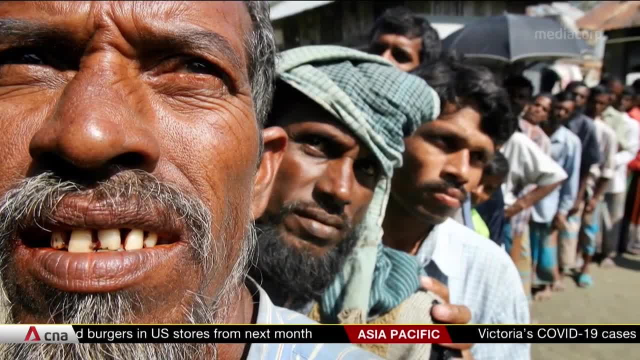 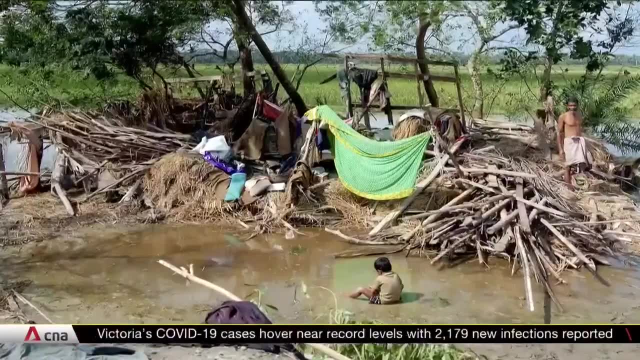 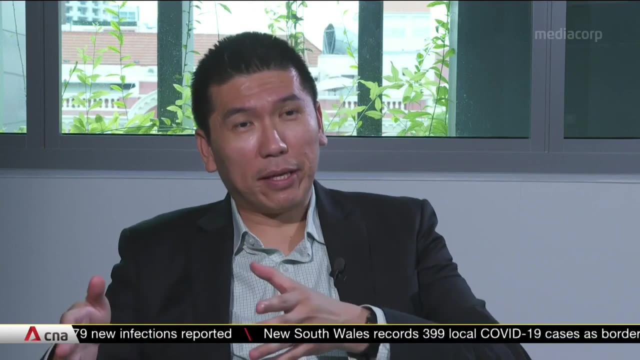 plan to move away when they are no longer able to continue where they are. but the sheer range and time scale of such adaptive measures makes it hard to predict consequences both intended and unintended. for instance, solar radiation management, which is one way of geoengineering hacking the planet to. 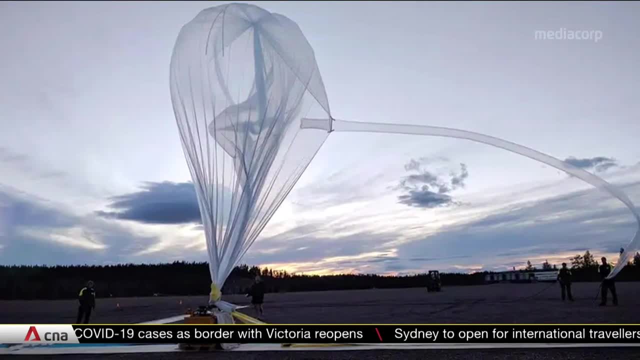 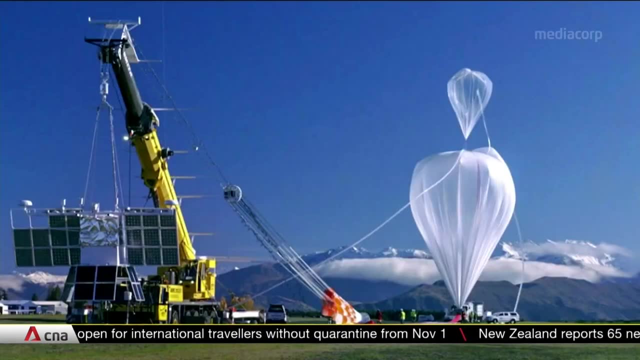 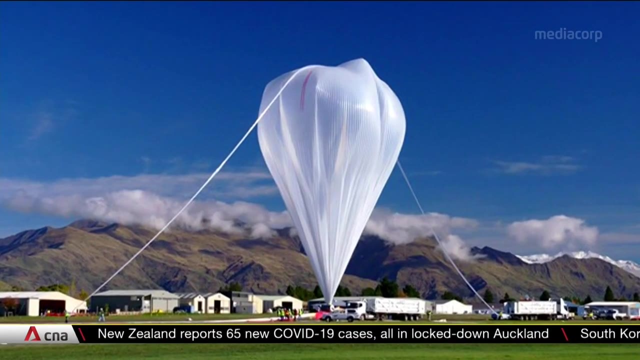 reduce incoming solar radiation, in other words, trying to cool a region by stopping the sun from reaching the surface. the unintended consequence is that very little thought goes into thinking about who maintains the amount of aerosols that are injected into the atmosphere for managing solar radiation. also, the 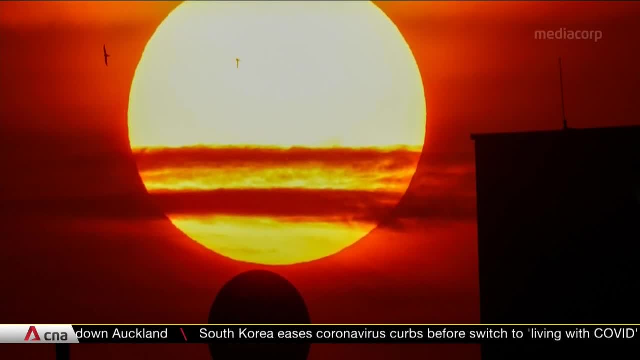 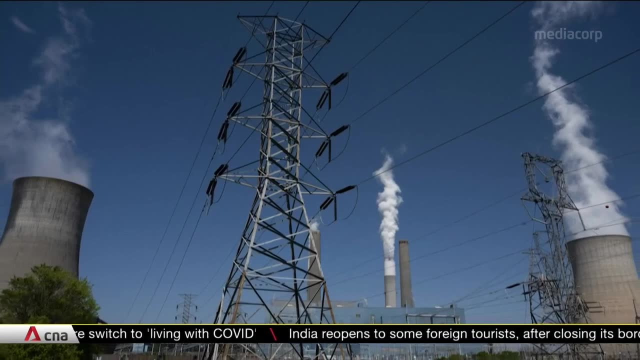 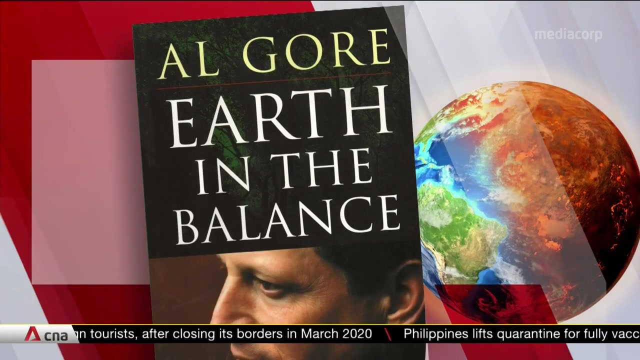 dependence on these sort of new technologies, like geoengineering, can often detract from the important you know need to cut the sources of climate change. it was this reluctance to detract from the task of mitigation that in the 1990s, would drive then US Senator and later. 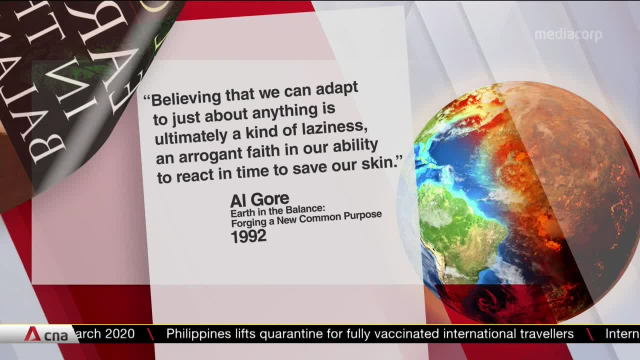 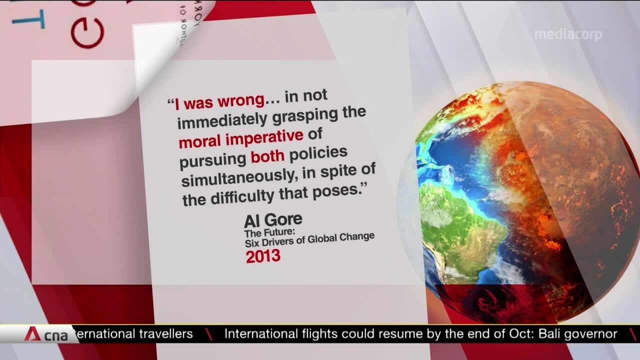 Vice President Al Gore to dismiss adaptation as a kind of laziness, a sentiment he would retract by the 2010s, admitting he had been wrong not to grasp the moral imperative of acting on both fronts. in the richer and, for now at least, the safer parts of the world, there is still the luxury of debate for countries like 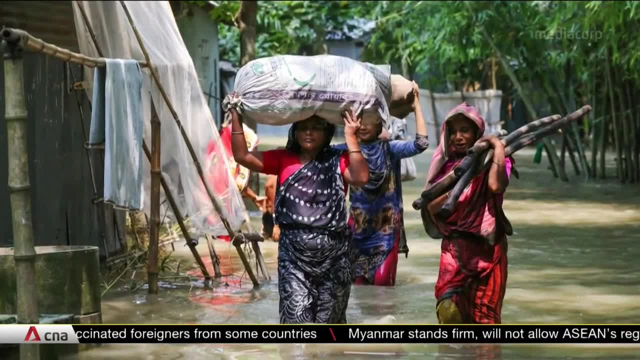 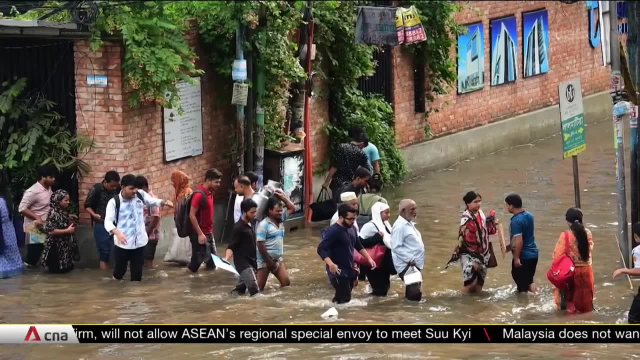 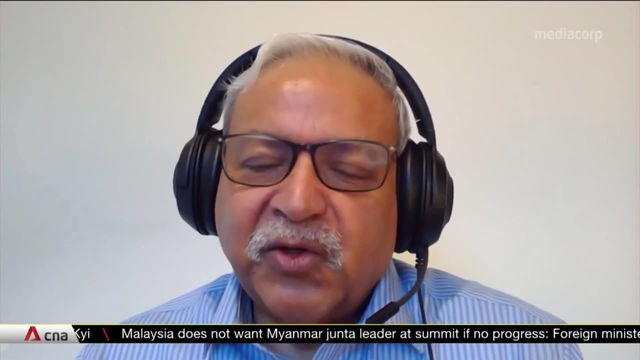 Bangladesh. the time to act was yesterday, just so they can keep their heads above water. for today. the whole world is going to have to adapt, whether they like it or not. Bangladesh is probably the most aware Society about climate change and we are preparing ourselves and what we do today, the 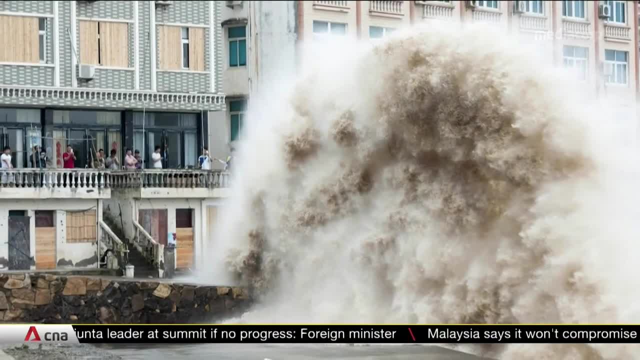 rest of the world is going to have to do tomorrow. there's no escape from this. climate change is right. it's going to get worse.